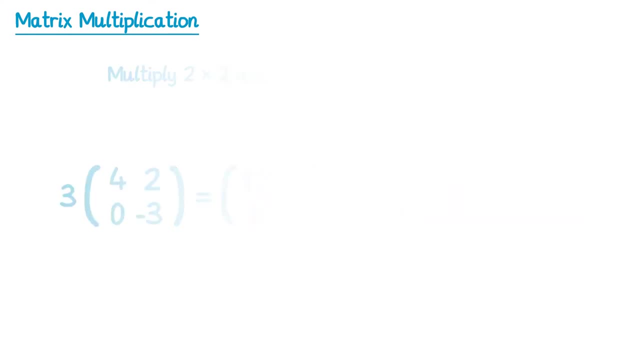 five times one, which gets you five. You also need to know how to multiply a matrix by another matrix. We're going to start by looking at how you multiply a two by two matrix by a two by one matrix. So let's take a two by two matrix and 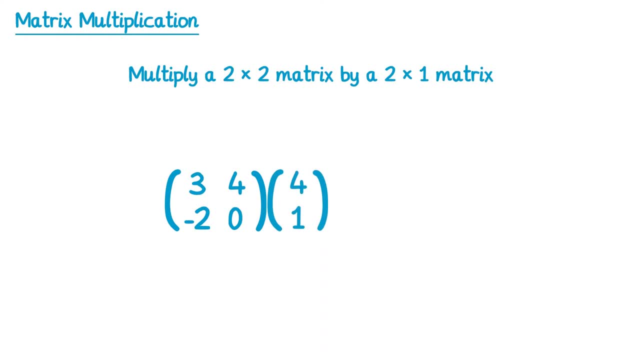 we'll multiply that by a two by one matrix, and you don't need to put a multiplication sign in the middle, you just write them next to each other like this: That means multiplied. Now, multiplying matrices can be a bit confusing at first. The more you practice, the easier it will become. What you 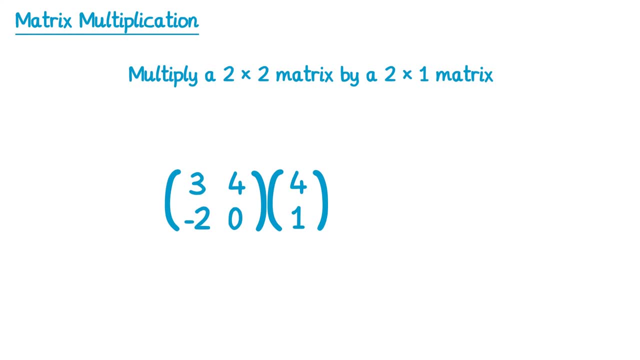 need to do is identify the rows from the matrix and then multiply them by a two by two matrix- The first matrix- and you pair them up with the columns from the second matrix. So we're going to start with the first row from the first matrix and we're going to match that up with the first. 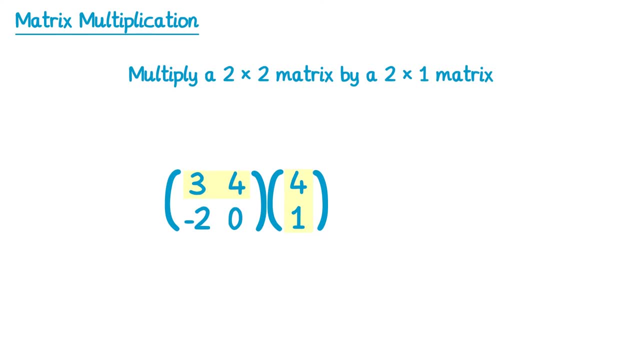 column. Well, there is only one column from the second matrix. The resulting matrix here will be another two by one matrix. So what we do is we look at this row and this column that we've highlighted and we match up the numbers. So the first one here, we've got three and we're going to. 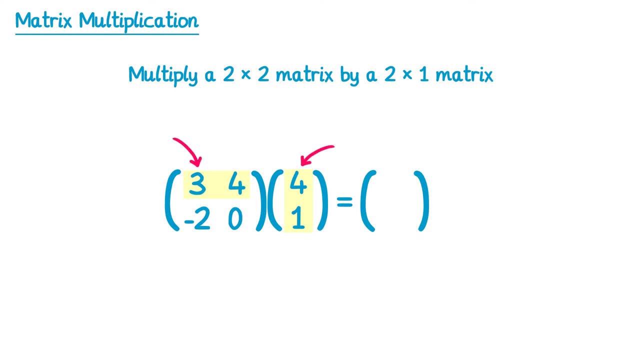 match that up with the first one on the second matrix, which is four, and you multiply these. So we do the same thing, but with the second numbers in each. So we've got four- that's the second number in this row- and one- that's the second number in this column. You do four times one. 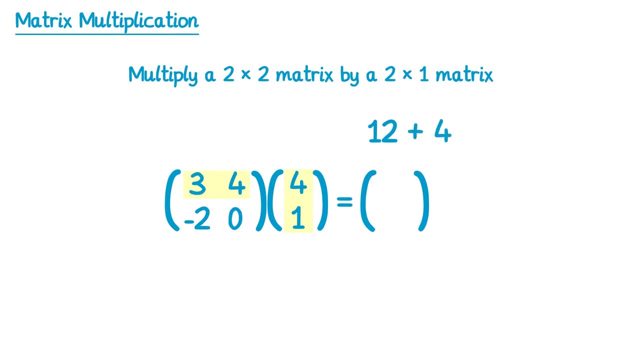 which is four, and you add that on. So we got twelve from the first multiplication, four from the second multiplication, and twelve plus four makes sixteen. You then repeat this process, but this time with the second row. So we've got negative two, zero, and we match. 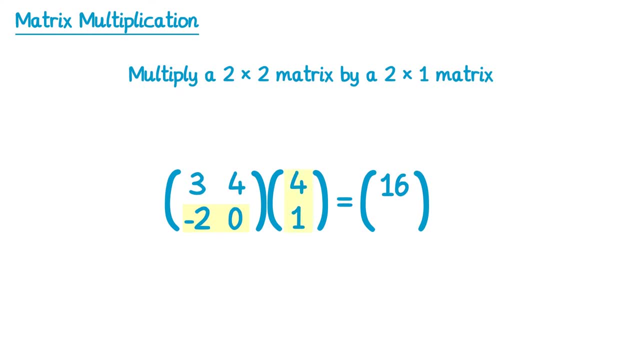 that up with the only column. we've got four one. So we did the first element so negative two times the four, which gets you negative eight. and then the second element, the zero here times the one, which gets you zero. so we add on zero, which of course gets you negative. 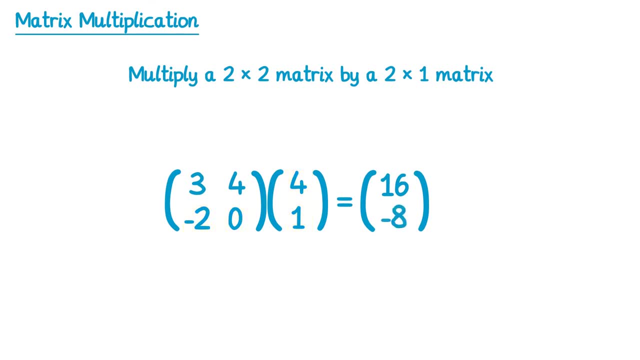 eight. So the answer is another two by one matrix, sixteen negative eight. Now you also need to be able to multiply a two by two matrix by another two by two matrix, and this is where things can get more complicated still. So let's take two two by two matrices like this: 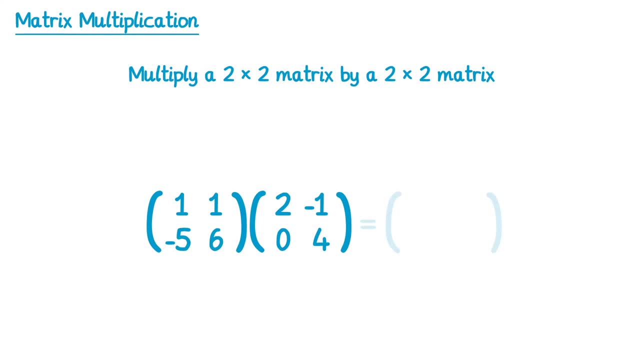 And the resulting matrix will also be a two by two matrix. So we start with the first matrix and select the first row and the second matrix. we select the first column And we'll do just as we did before. so we'll do one times two, which is two, and then we'll add to that. 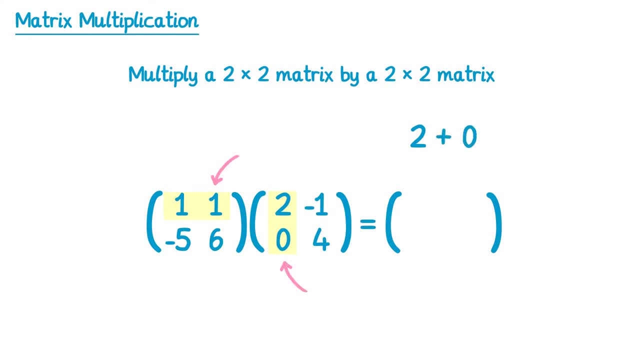 one times zero, which is of course zero, and two add zero makes two. Now, this time we'll start with the first row again, but move on to the second column. So we do one times negative 1, which is negative 1, and then this second one here times 4, which gets you plus 4, and negative. 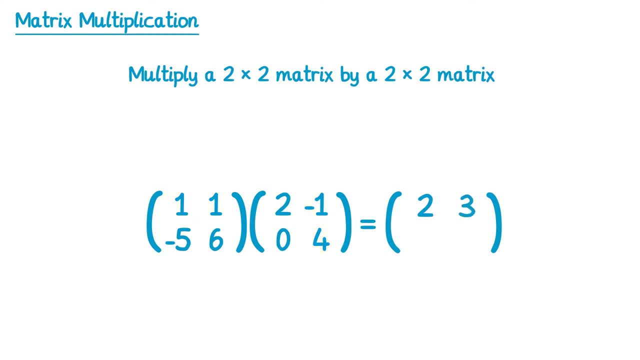 1 plus 4 gets you 3.. We now move on to the second row. so negative 5: 6 here, but go back to the first column. so negative 5 times 2 gets you negative 10, and then 6 times 0 is plus 0. so we end up with 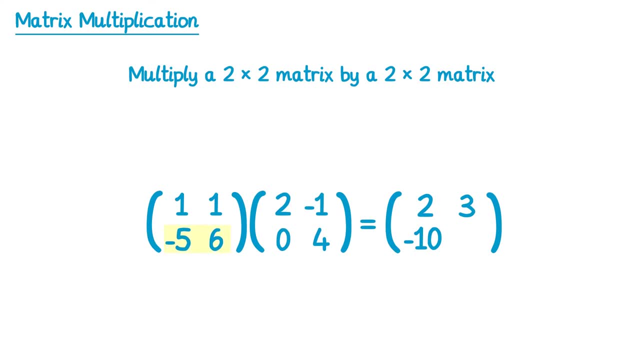 negative 10.. And finally, we do the second row times, the second column. so negative 5 times negative 1, which is a positive 5. and then we add to this 6 times 4, which means add 24, and 5 add 24. 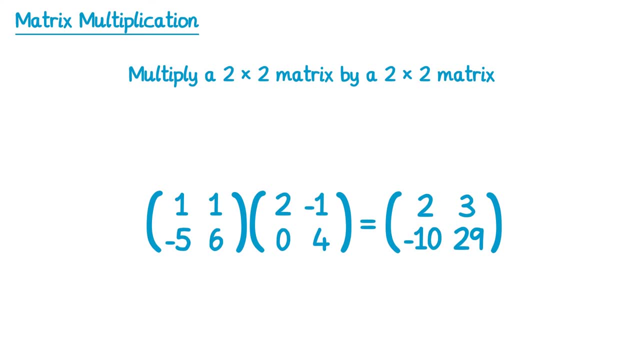 is 29.. So this is your answer. The next thing you need to understand is that, in general, matrix multiplication is not commutative. The word commutative concerns the all-in-one matrix multiplication. The word commutative concerns the all-in-one matrix. 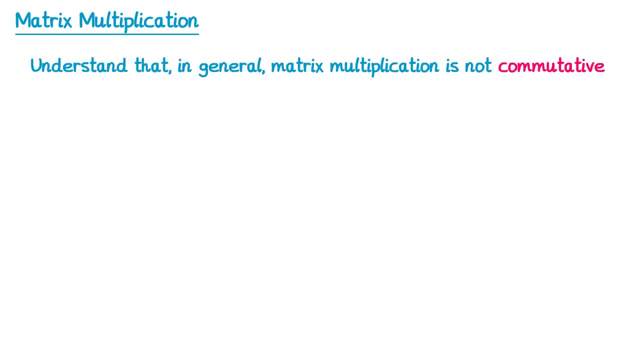 order in which you multiply. So if we take regular multiplication like 5 times 4, which equals 20, this is commutative, because you can change the order like 4 times 5 and get the same result. Unfortunately, this doesn't apply to matrices, and I'll show you why. now Let's take 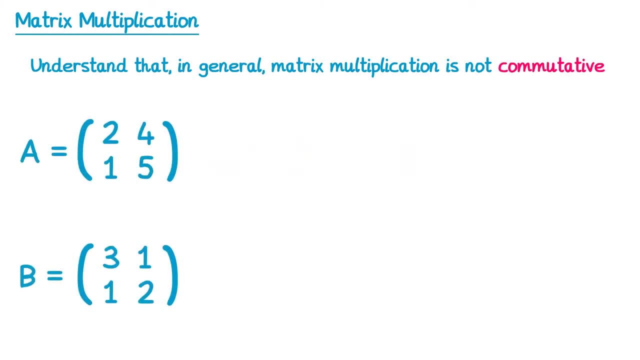 two matrices, so matrix A and matrix B, and we'll first of all do AB, which means we start with matrix A and we multiply it by matrix B. This will give us a 2x2 matrix, like we practiced previously. so we'll do the first row multiplied by the first column. so 2 times 3 gives you 6 and 4 times 1. 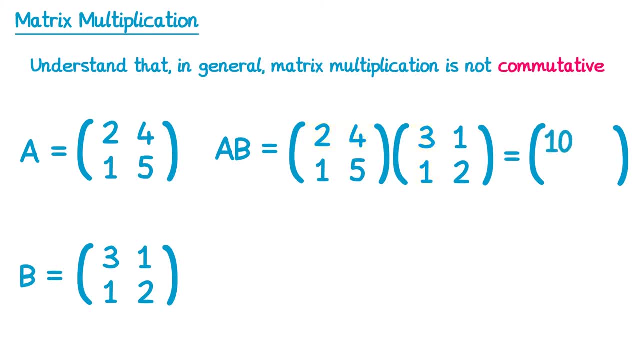 gives you 4, and then we add the 6 and 4 to get 10.. We then stick with the first row but multiply by the second column. so 2 times 1 is 2, and 4 times 2 is 8, and 2 add 8 is also 10.. We then move on to. 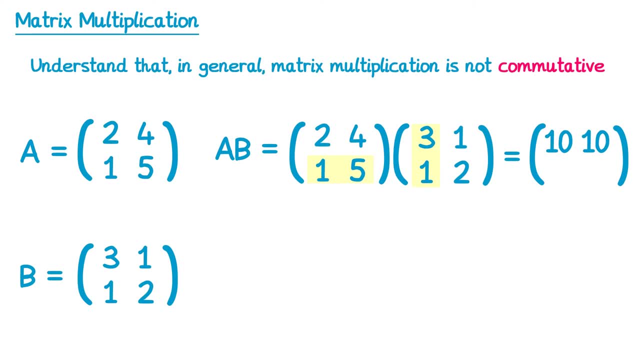 the second row with the first column. so 1 times 3 is 3, 5 times 1 is 5 and 3 add 5 is 8.. And finally, the second row with the second column: 1 times 1 is 1 and 5 times 2 is 10 and you add those. 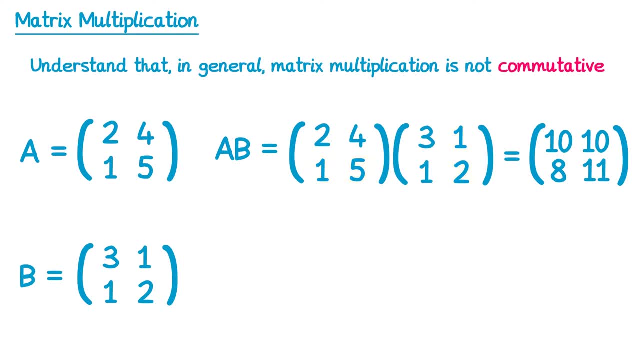 together and you get 11.. Now what if we reverse the order? This time we'll do BA, so we'll start with matrix B and multiply by matrix A Again. this will give us a 2x2 matrix, so we'll do 3: 1. 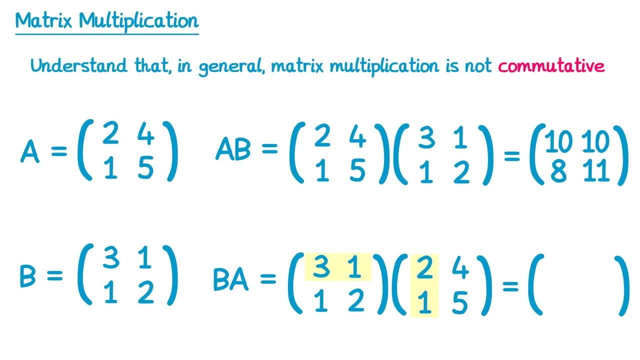 multiplied by 2, 1, 3 times 2 is 6,, 1 times 1 is 1 and 6. add 1 gives you 7.. 3, 1 multiplied by 4, 5, 3, 4s are 12, 1, 5 is 5, add 12 and 5, you get 17.. Then 1, 2 times 2, 1,. 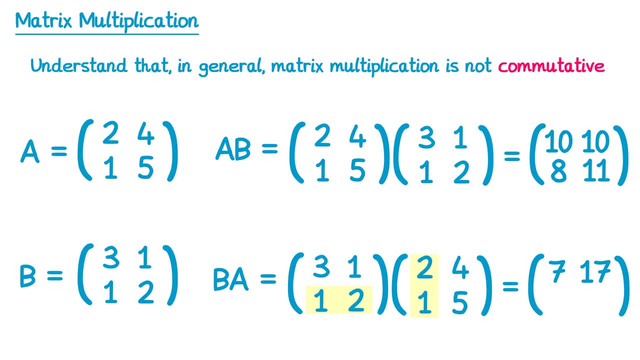 so we have 1 times 2, which is 2, and 2 times 1, which is also 2, so 2 add 2 is 4.. And finally, 1, 2 with 4: 5, 1 times 4 is 4 and 2: 5s are 10, 4 add 10 is 14.. 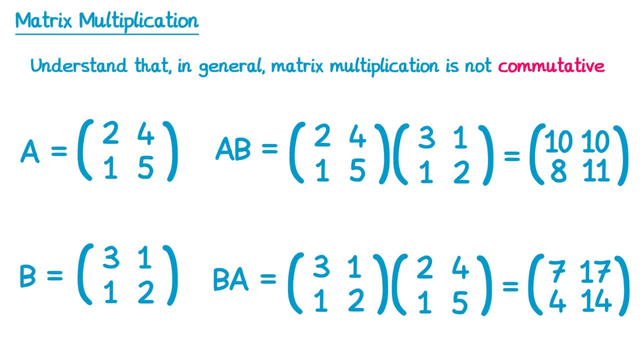 You can see from this that the results of AB were not the same as BA, and this shows us that multiplication is in general not commutative. There will be some examples where this does work, but to be commutative it needs to apply to all cases. 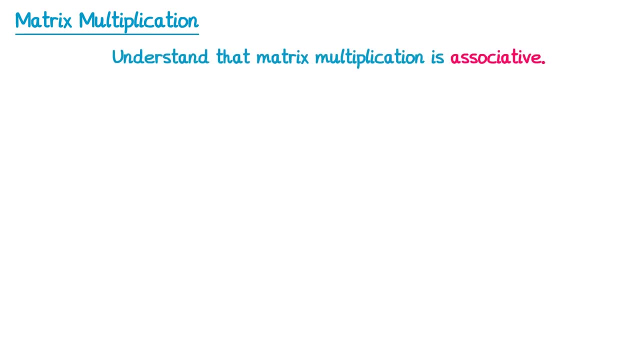 The final thing that the specification asks you to know is that matrix multiplication is associative. Now again, if you don't know what associative means, I'll show you with an example. If you take 2 times 5 times 6, this gives you 60. Now you could do this by: 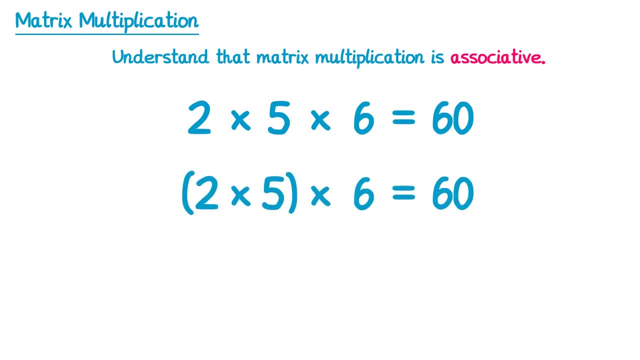 doing 2 times 5 first, which is 10, and then times that by 6 to get 60, and also do 2 times 5 times 6 to get 60. Then again you could do the same thing with 2 times 5 and the same.